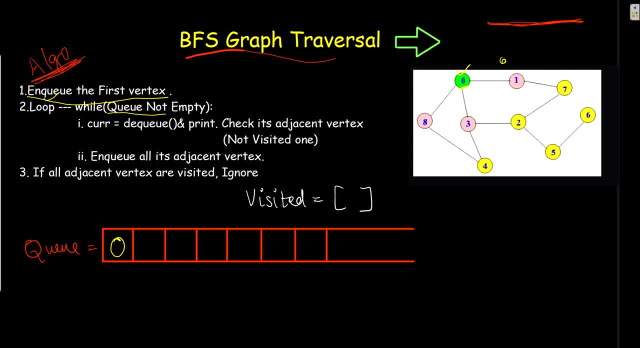 Then, secondly, it will check whether Q is empty or not. Here Q is not empty, So it will go inside the while loop And it says dequeue. So I will dequeue zero and will put into current, as it should be allocated to the current variable. 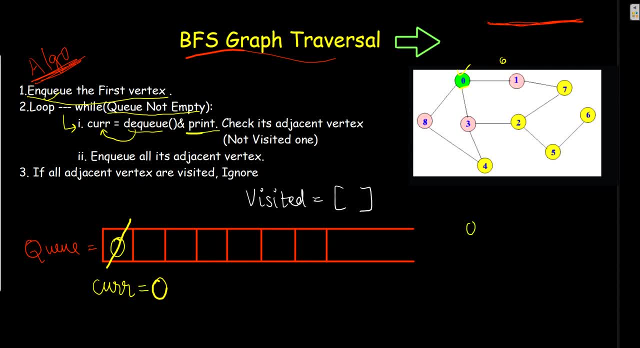 And it says to print. So here I'll be printing for BFS: zero will be printed, zero in visited also. as I have visited zero, I'll put tick also for my convenience And with that I will also fill in visited so that i can remember which node has been visited. so zero is in visited array, then check its. 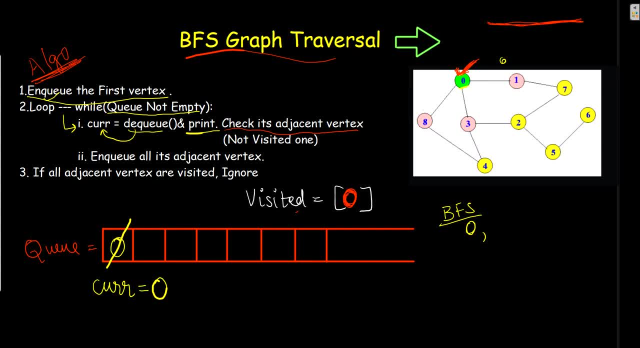 adjacent vertex. so for zero we have adjacent eight, three and one. adjacent vertex will be which are first connection of our vertex. so eight, three and one which are not visited, as we don't have eight, three, one in visited, so enqueue all its adjacent vertex. so here i will enqueue eight, three and one. you can either fill 8, 3, 1 or 138 or 381, whichever. 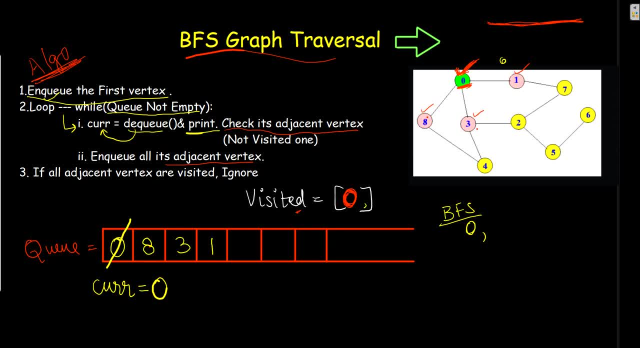 order you want. with that i will also fill this 8, 3, 1 in visited, because we have visited eight, three, eight three and 1 again. it will go to y loop and will check whether q is empty or not. so here we can check q is not empty. here we have three elements. so it says to dq and put into current. so now we have. 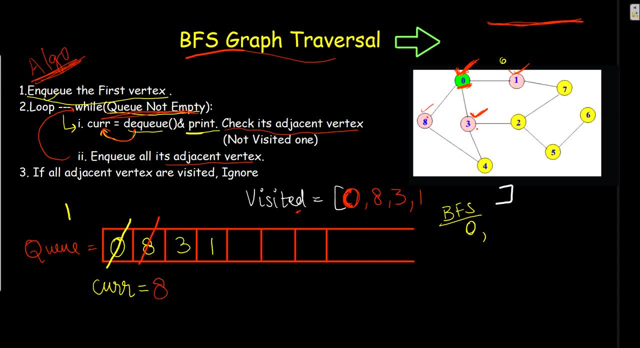 8. as q always works on fifo first in, first out, so first is right now 8. so here we got in current 8, then print it. so here i will print 8, then check its adjacent vertex. so for 8, if i check we have 0 and 4, but 0 is already there in visited. 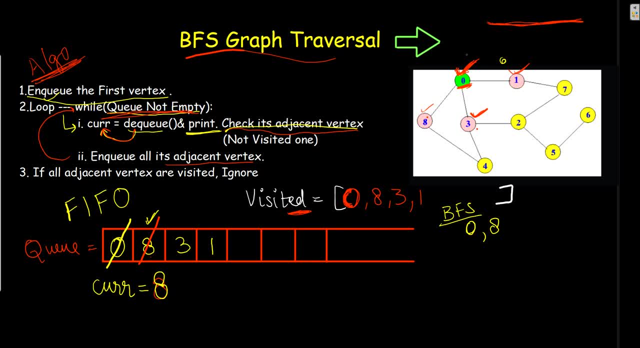 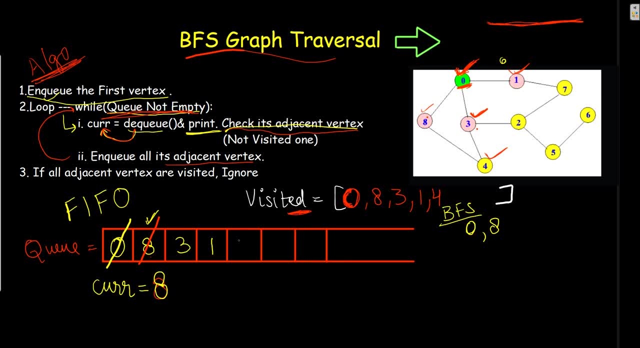 as this is now visited and will put into my q. then again it will go to y loop and will check whether q is empty or not. here in q we have 3 elements. it's not empty so it says to dq the first element, which is 3. so it will dq and will. 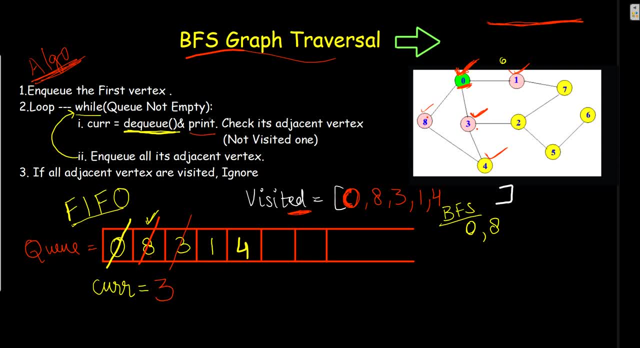 put into current, then print it. so here i will get 3 also, and then i need to check its adjacent vertex. so for 3 i have 0, 2 and 4, out of which 0 and 4 are already visited. as we can see here we have 0 and 4, but for 2 it's not there. so i'll take 2 and will put into visited. 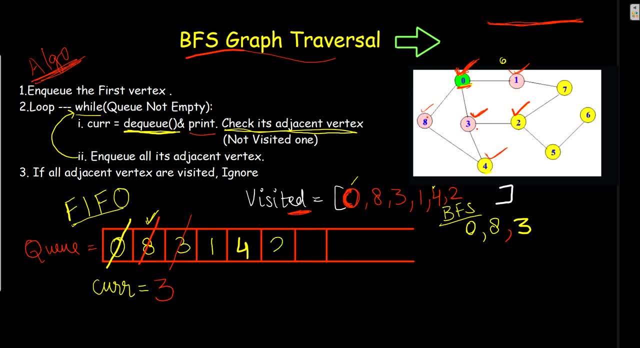 as it is not visited. so i will enqueue 2 here. then again it will go to y loop and check whether q is empty. no, it's not empty. so again i will dq 1 and will put into current with that. i will print then for 1. i will check the adjacent vertex. it's 0 and 7, out of which 0 is already visited because 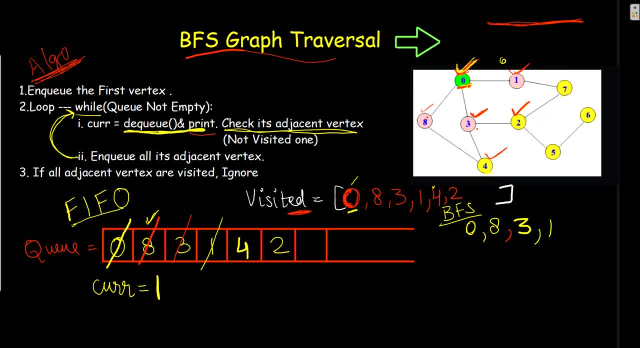 we haven't visited 0. now i need to take 7. so i will take 7 here and will enqueue. then again it will go to y loop and will check whether q is empty. no, it's not. so again it will dq the first 4 and will put into current. then it will print also as it says dq and print then for 4 it will. 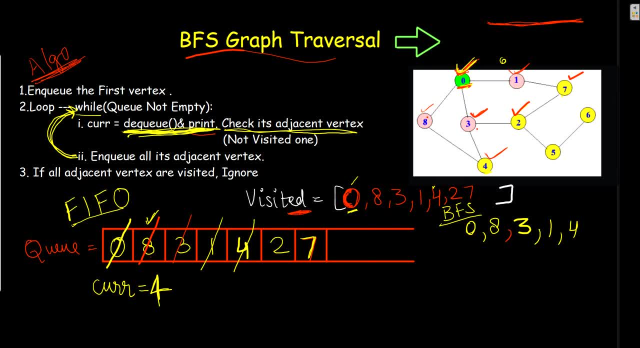 check its adjacent vertex 4. we have 8 and 3 which are already visited. so here the third point comes. if all adjacent vertex are visited, ignore. so i will ignore here. then again it will go to y loop and will check whether q is empty. q is not empty. here we have two elements, so it will dq and print. 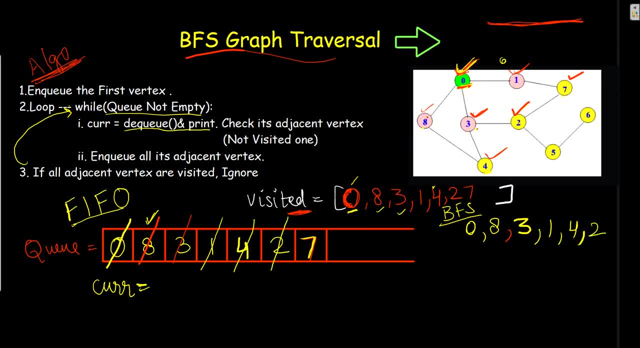 the first element, 2, and in current we have 2. now we will check for 2. adjacent vertex it's 3, 7 and 5, out of which 3, 7 are already visited. so we need to take 5 now, write 5 and will enqueue now again it will go to y loop and will check whether q is empty. no, it's not. 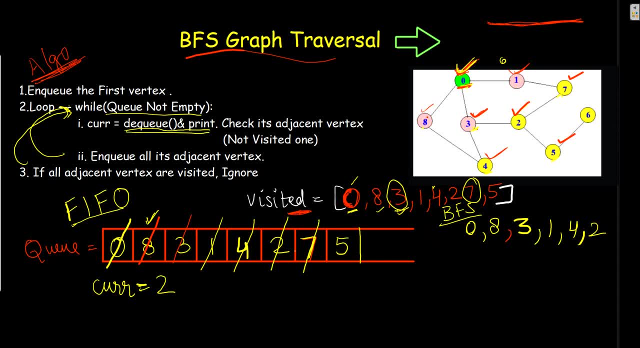 so it will dq the first element, which is 7, and will print and will put into current. now for 7. it will check the adjacent vertex. it's 1 and 2, out of which both are visited. so it will ignore here and again it will go to y loop and will check whether q is empty. no 5 is there. so for 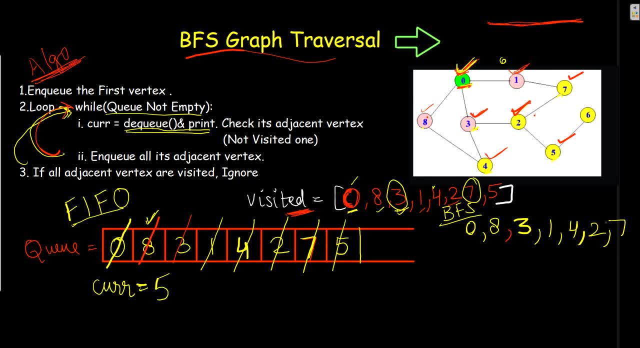 5, it will dq and will print over here. then for 5 it will check its adjacent vertex, its 2 and 6, out of which 2 is already covered in visited. so it will check for 6 and will enqueue here and will also put into visited. then again it will go. whether q is empty now. no, it's not because we. 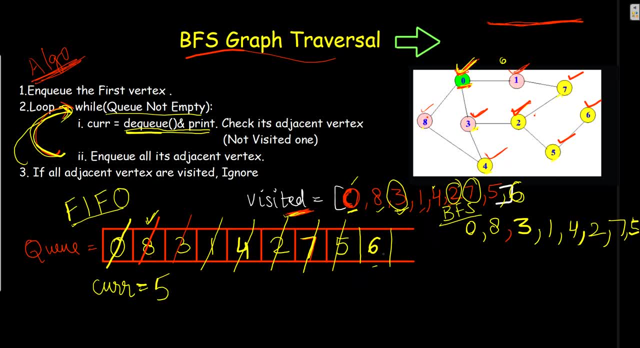 have 6 over here. so again it will dequeue 6 and will put into current and will also print 6. then it will check for 6 whether it has any non-visited adjacent vertex. 6 has only 5 which is already visited. so again it will go and will check into while loop whether q is empty now. now q is empty. 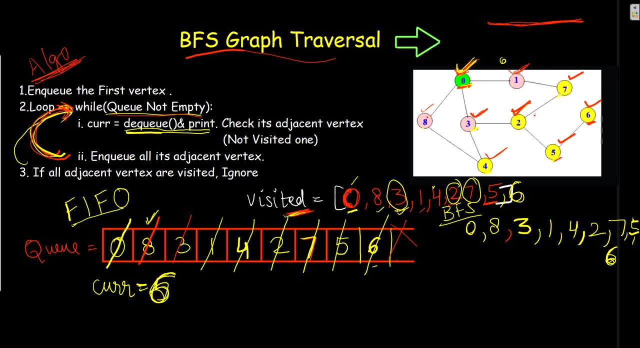 as we don't have any element over here, so it will come out of the while loop. and here we got 0, 8, 3, 1, then 4, 2, 7, 5, 6 horizontally right. so this is all about pfs, bfs. we are making use of q, which works on first in, first out. so here we'll be making use of q. 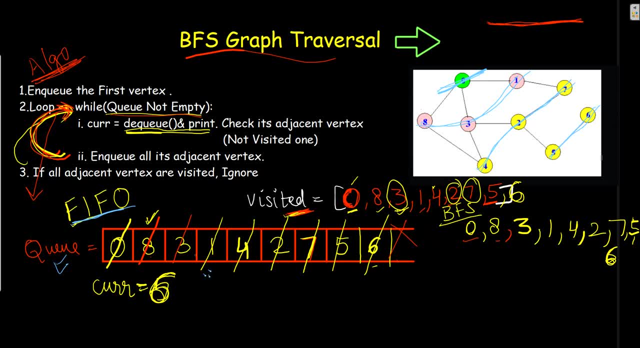 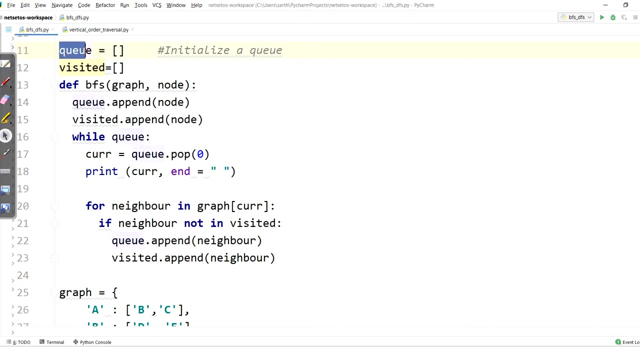 and we'll check whether q is empty or not. till q doesn't get empty, we'll be enqueuing its adjacent vertex, which are not visited. so let's see its implementation, how it works in python. so here we have a program for bfs where we have taken q and visited array as an empty. let's see it. 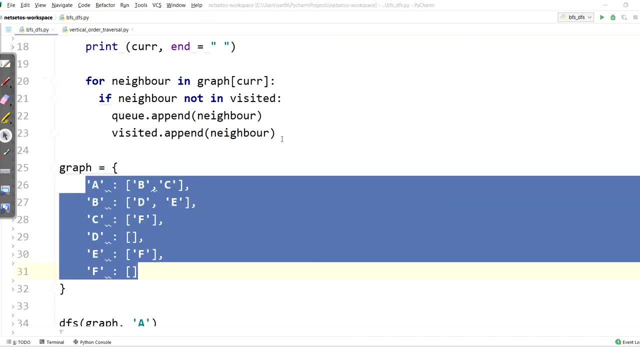 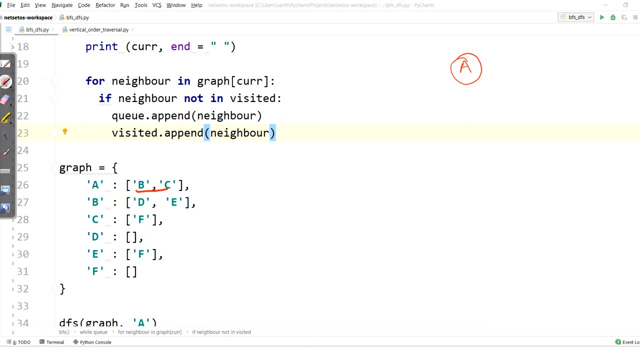 by taking this example. so first of all i'll plot this, which says a, which is connected to b and c, so what i'll do? i'll make use of b and c. then it says b is connected to d and e, so here i'll take d and e. c is connected to f, so here i'll connect c with f. d is empty, so here. 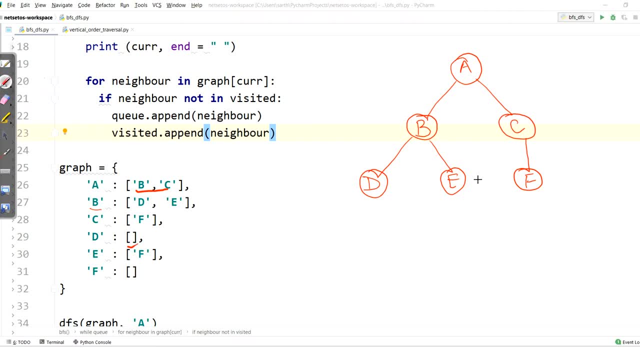 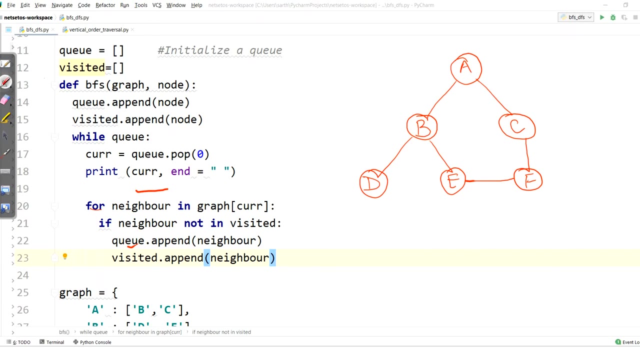 i won't be connecting d. then e is connected to f. f is empty. so this is our graph. on the basis of this graph, we'll be working for our code. let's see how it works. first, q is empty, so here i'll take q. let me draw q over here and we'll take visited and array. 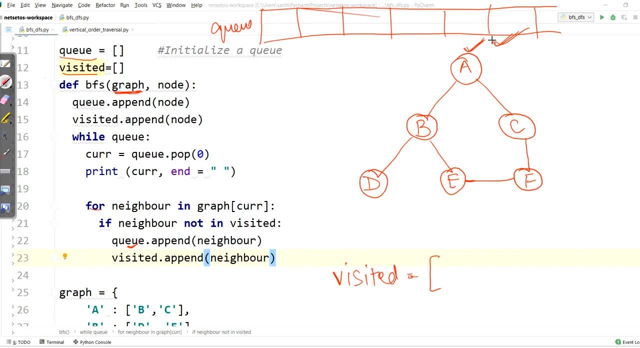 now here, graph. we have taken this as an input parameter because we'll be providing this graph on which we have to code. then we have node, the first vertex. we can start with any of the node whichever we like. here i'm starting with a node. now it says first append node into q. so here q is an array. so for adding any node, 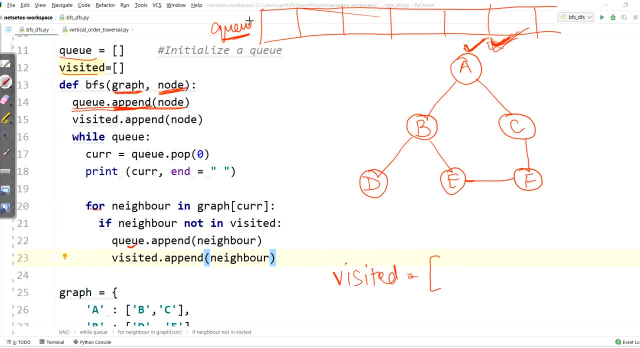 to an array we make use of append. so here i took node which is a and i also appended node a, visited. then it says: while is que empty, this means work Q get empty. So here Q is not empty, as we have A over here, So it will go inside it and will pop. 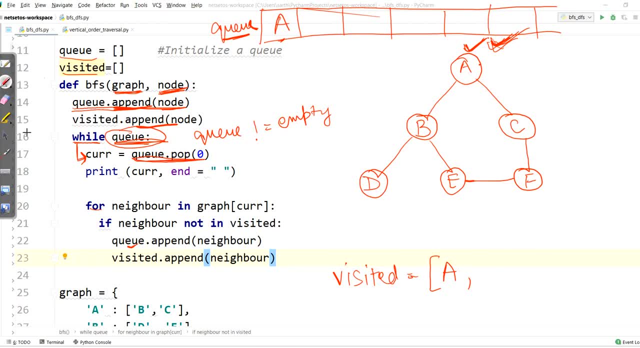 first element of Q, as Q always works on FIFO right. So here in current I will have A, the first element. Either I can cut or I can delete it. Here I am cutting Here. I don't have any element in Q right now. It says print current. So here I will write whichever element has to be printed. So I 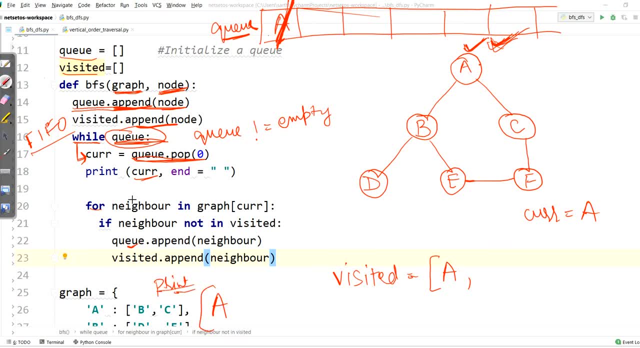 will write print: Okay, Then I will apply a loop for neighbor for adjacent vertex In graph current on the basis of current. if neighbor not in visited, it says is neighbor to be taken which are not in visited. So here it has B and C. B and C are not present in visited array, So append in Q. So here B and C. 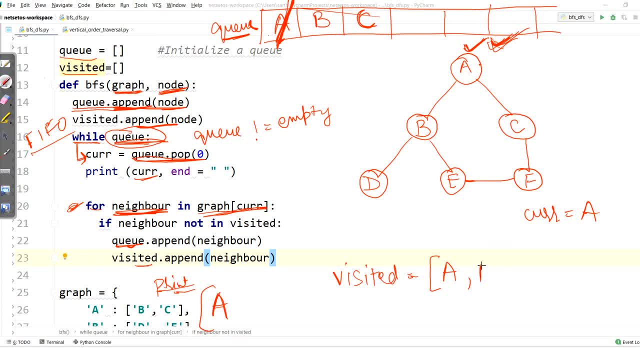 will be appended and also visited, will have B and C. Then again it will check while Q is empty. now Q has B and C. So here it will pop out the first element, which is B and C. So here it will pop out B is B and will print: then it says: to check B's neighbor, which came out in current. So for B, 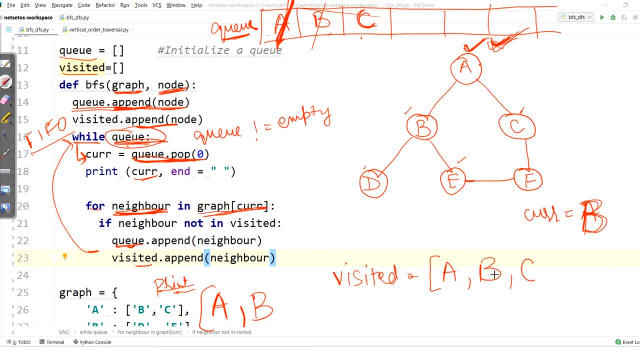 neighbor is D and E. D and E are not in visited, So I will append D and E in Q and also in visited. Now, do D and E are visited? Then again, it will to, while it will check whether q is empty. no, we have three elements: c, d, e. then it says: 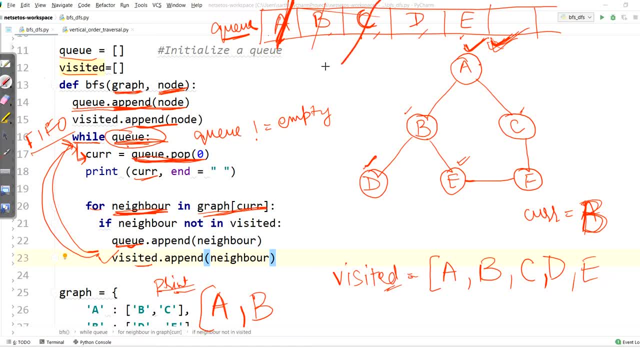 to pop first element, which is c, and will put into current. so in current we will have c. then it will check c's neighbor. c neighbor is a and f also it says it should not been visited. a is already there in visited, so we will take f and append in q and also in visited. so here we. 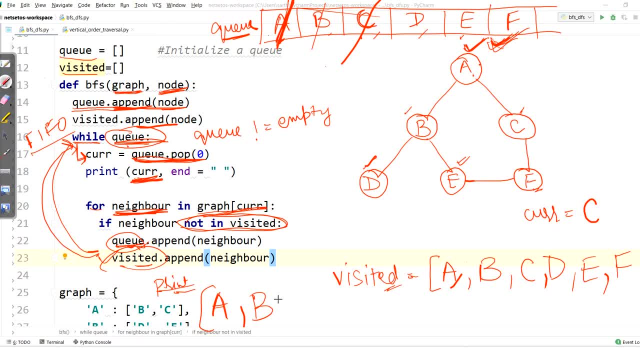 will have f also and also- i forgot this- c will be printed. whichever current element will be there will be printed over here. let me delete this. then again, it will go and check whether q is empty. we have d, e and f, so so. so so current will have the first element of q, which is d, and will get printed. 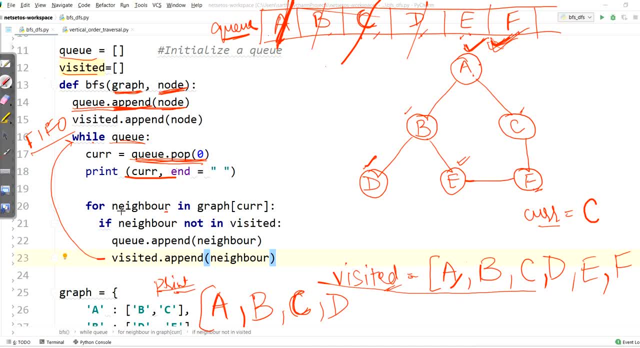 right, then it will check its neighbor. d's neighbor are b only, which should not been visited. so here b is already printed, so it won't be going here and will directly go to while loop and will check whether q is empty. now e and f are there. 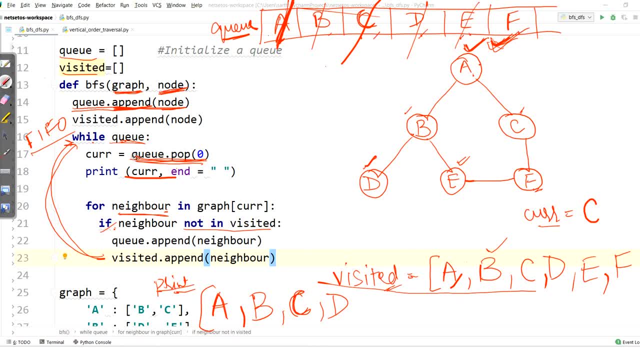 so it will pop first element and will put into current. so here we will have in current: e and e will be printed as it says here. then it will check its neighbor. e's neighbor is f and b. b is already visited, printed and also f is printed as we have. it is visited. so it will pop first element and will 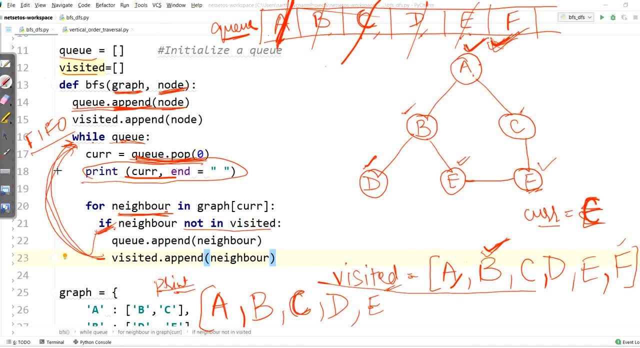 be printed. as of now it won't be going inside this f and directly will go to while loop and will check whether q is empty. no, we have f over here. so it says to pop the first element, which is only element. so here i will take f in current and printed. so here it will be printed. then it will check whether f has any neighbor. f has c and e. c and e are already there. then we will check whether f has any neighbor. f has c and e. c and e are already there. 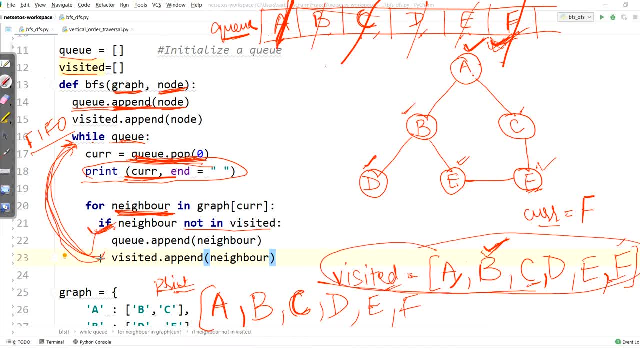 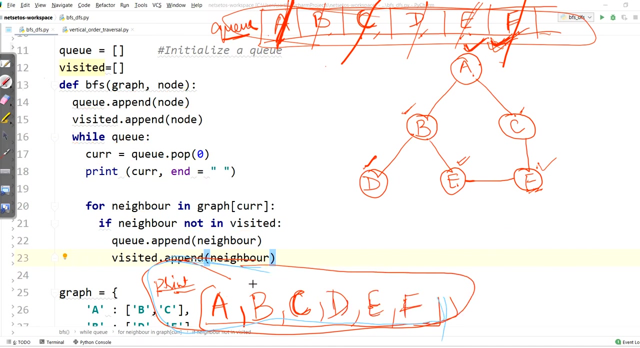 already there. it visited. it won't be going inside if and we'll go to while loop and this time it will check while q is empty. now, yes, now q is empty, as all cuts are there. there is no element in q, so it will print a, b, c, d, e and f. now, if we see it closely, first a is printed, then b, then c. 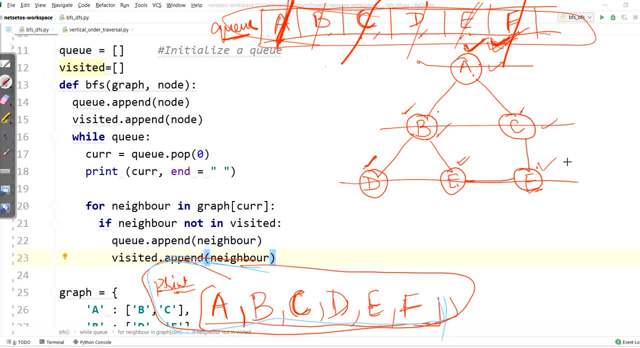 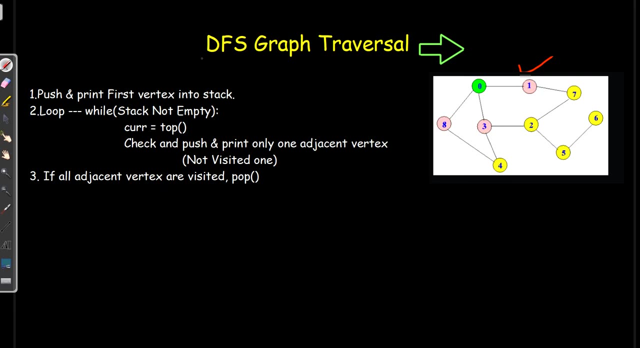 a, b, c, d, e, f, which is in horizontal. this is all about bfs: breadth first search. now let us see depth, first search. so here we'll be making use of same graph which we took for bfs. so here we'll start and here we'll have stick in bfs. we took q now for dfs. 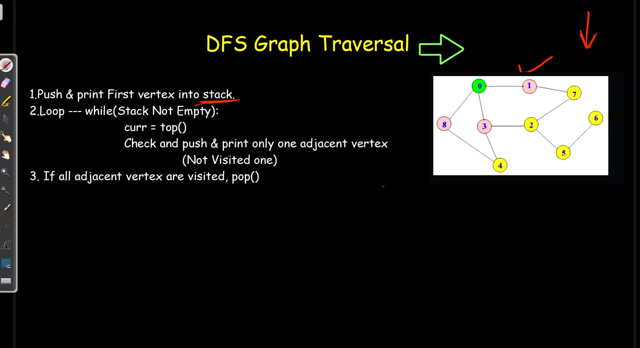 first search, which is in vertical, so I'll draw stack over here. so this is our stack and stack, as you all know, it works on leaf form. last in, first out. so here I'll also take visited array so as to track which elements are visited one, because we won't be taking 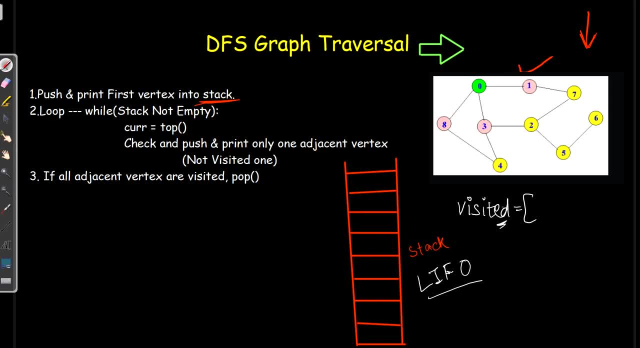 the nodes which are not visited we'll be adding into a stack. so let's start first. it says to push and print the first vertex into stack. so here also it depends on you. whichever vertex you want to start with you can take. here. I'll start with zero, so for zero I'll enter the first vertex, zero. 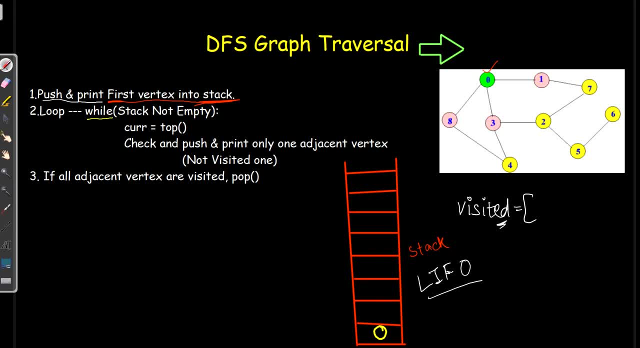 in the stack. then it will go into while loop and will check whether stack is empty or not. stack is not empty because we have zero in our stack. so it will go inside while loop and will have the top most element of stack which is zero, and will fill in current. so in current we have zero. then it says: 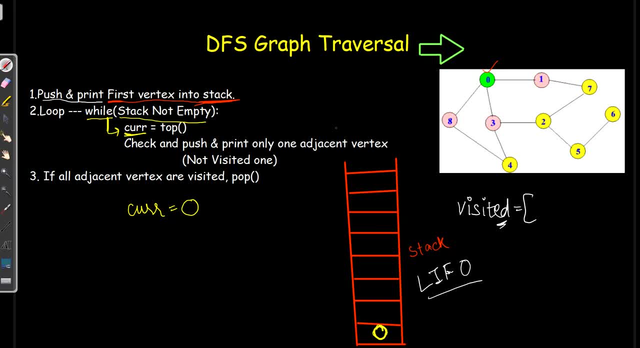 check and push and print only zero. one adjacent vertex in queue. we used to take all vertexes. here we'll be taking just one for zero. we have eight, three and one. we can take any of them. I'll take eight. first of all, I need to print. 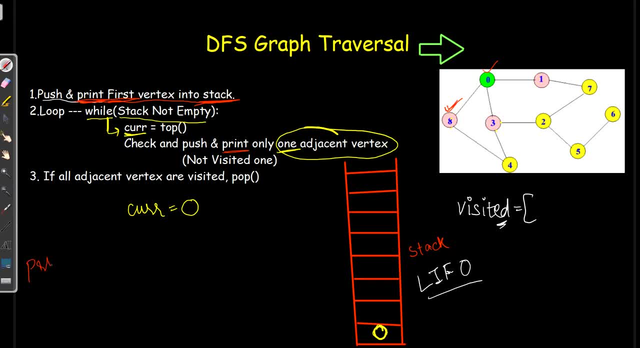 the first vertex. so here I'll take all the elements which I need to print. so first element was zero, as it says here. then I'll take all the elements which I need to print. so here I'll take all the elements which I need to print. so here I'll take all the elements. here it says: push only one adjacent vertex. 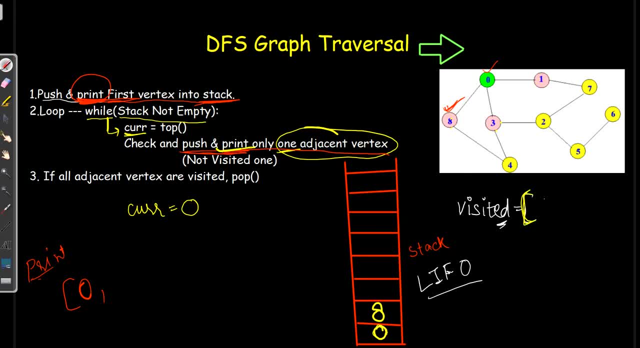 here it says: push only one adjacent vertex. so I'll push eight in my stack and also print. I will take zero first. so I'll push eight in my stack and also print. I will take zero first. then here I will check whether eight is visited. here it is not visited, as I don't have eight here. so here I'll put eight and will print here. so eight will get printed, as it is not visited one. 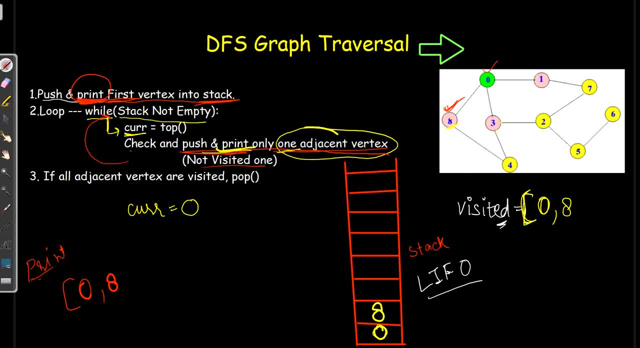 then again it will go to while loop and will check whether stack is empty. stack is not empty, so here it will go to its top 8. allot this 8 to current. then it will check whether 8's vertex, the adjacent vertex for 8, are 0 and 4, out of which 0 is already visited. we have 0 over here. 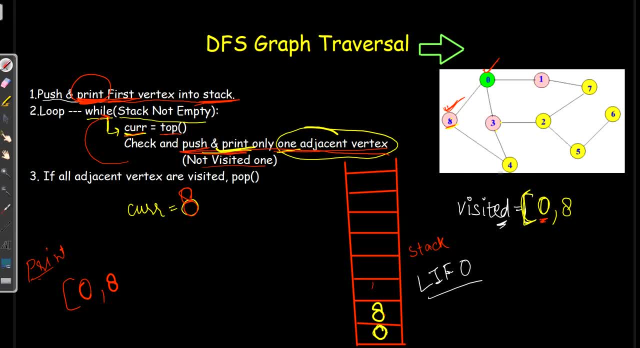 so it will take 4 and will push into the stack right, and also it will print only one vertex, which is 4, as it is a not visited one. so here i will put 4. now 4 is visited one. then again it will go to while loop and will check whether stack is empty. no, its stack. 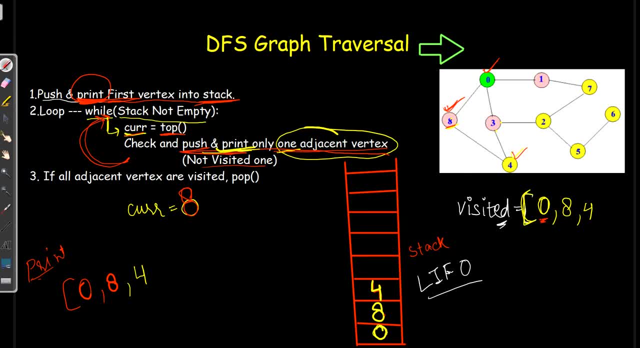 is still not empty. so it will take the first element. so it will take the top most element, 4. so here i will take 4 in my current and will check the adjacent vertex of 4. 4 has 8 and 3, out of which 8 is already visited, so we have just left 3. 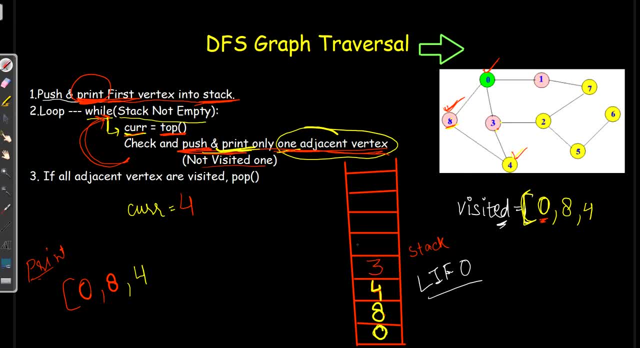 so i will push first 3 here, then print 3 here as 3 is not visited, and will put it as visited, right. then again it will go to while loop stack is not empty, so it will take the top most element, which is 3, into current. then it will check the 3's adjacent vertex, which are: 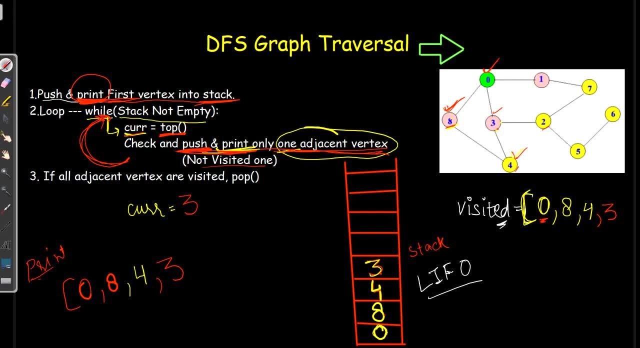 0 4 and 2 0 4 are already visited. 2 is not visited, so we will first push 2 in stack, then print. as it is not visited one now, we will make it visited one. then again it will go to while loop. 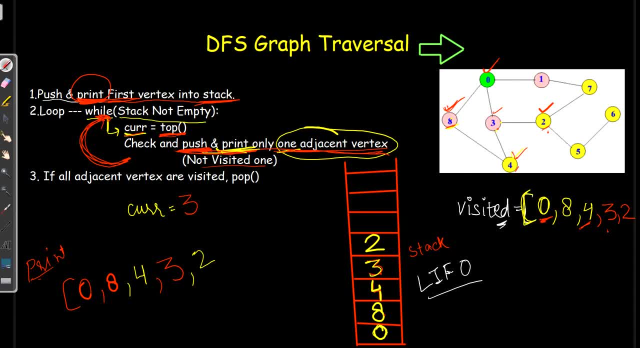 stack is not empty, so we will take the topmost element, which is 2, and will allot to current variable. then we will check 2's adjacent vertex, which are 7, 5 and 3, out of which 3 is already visited. now, out of 7 and 5, we need to take 1, so we can take any one of them. here i am taking 5. 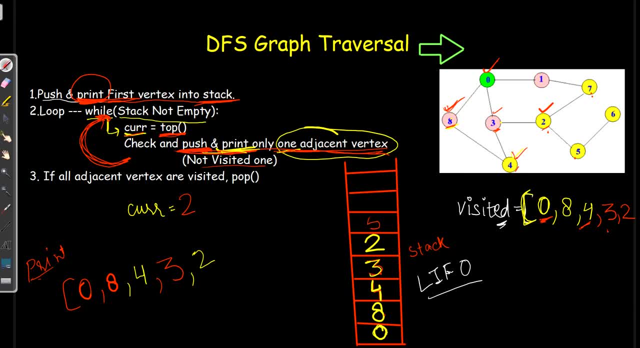 so first i need to push into stack, then print only one adjacent which is not visited. let's make it visited this time. then again it will go to: while loop stack is not empty, we will take the topmost element, which is 5, and will check the adjacent vertex for 5 it's 2 and 6- 2 is already. 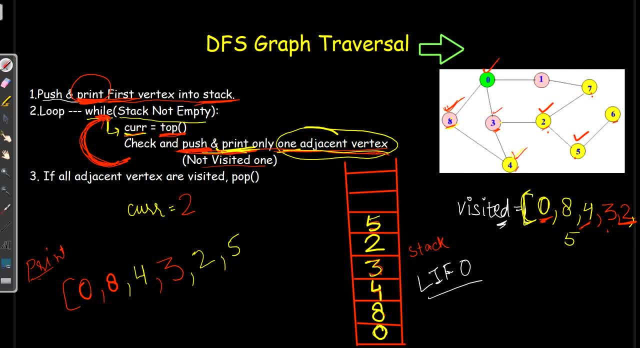 visited. so now we will take 6. first we will push into the stack, then print which is not visited. now we will make it visited one. then again it will go to while loop stack is not empty. so it will take the topmost element, which is 6, to the current. now current has 6. so for 6 we need to check the adjacent vertex. 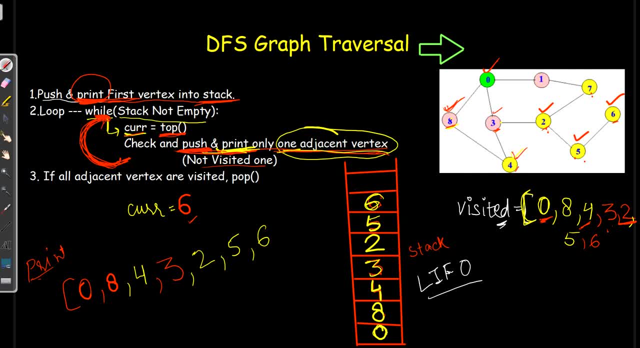 which has 5. but what can i see here? 5 already visited. so what i'll do if all adjacent vertex are visited? pop our element from the stack. so i will pop 6 now. now here left 5. now i need to check for 5, for 5. 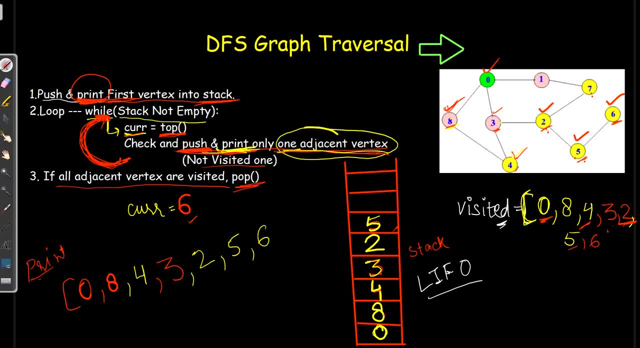 we have 2 and 6, the adjacent vertex. again, we will check the third instruction which says: if all the adjacent vertex are visited, pop a element from the stack. 2 and 6 are already visited. so what i'll do? i'll pop one element from here. now left is 2, so here i'll go to 2 and will. 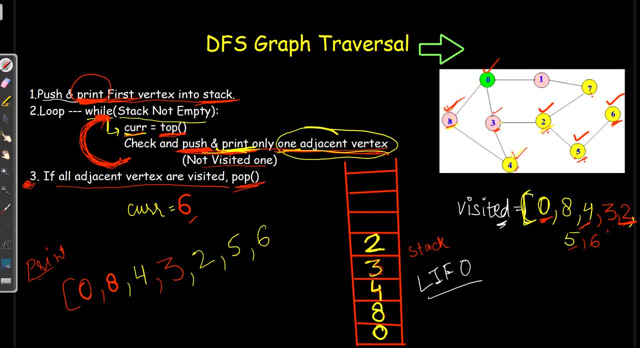 check the adjacent vertex for 2 now. now for 2. i will again go to while loop. stack is not empty. it will take the top most element to the coим over. therefore we need to check that olan is not empty. now here i will go to while loop and we'll check the tenho one you now like in the other case, the. stack is not empty and it will be exiting to here again will Set this universe to 7 and for now we will use a value, 0, and also like set to 0, which can take at the purpose of dividing the step side. and now we need to check the limit of state between the two elements, because twine Dialogues 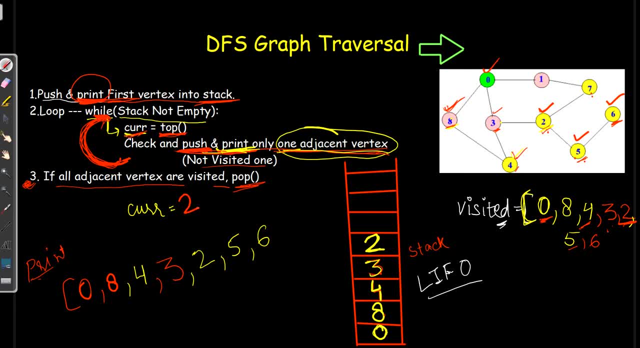 we will take the allein element from stack and shift it to the left side and set the령 which are into current here i got two in my current. now it will check for two. the adjacent vertex are three, five and seven. three and five are already visited, so we will take seven and we'll push into. 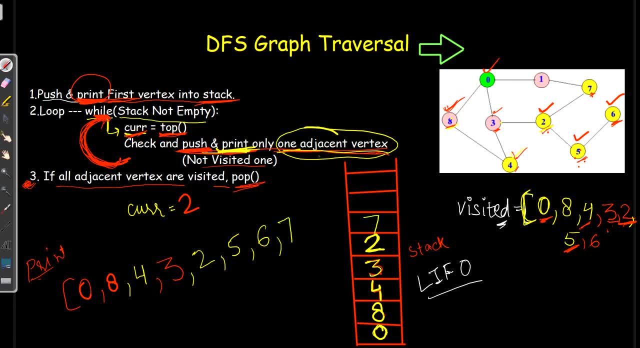 stack, then print it and we'll make it visited one. i'll enter here. then again it will go to while loop. is stack empty now? no, stack is still not empty. so it will take the topmost element, which is seven, and will put into current. so here current has seven element. then it will check the adjacent. 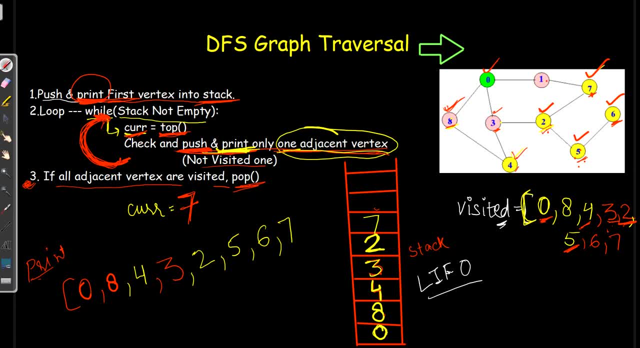 vertex for seven is two and one tool is already visited. here we have two in visited array. one is not visited, so first i need to push into stack, then print. as it is not a visited one, so let's make it visited one, as i will enter into the visited. then again it will go to while loop and will check whether stack is empty. 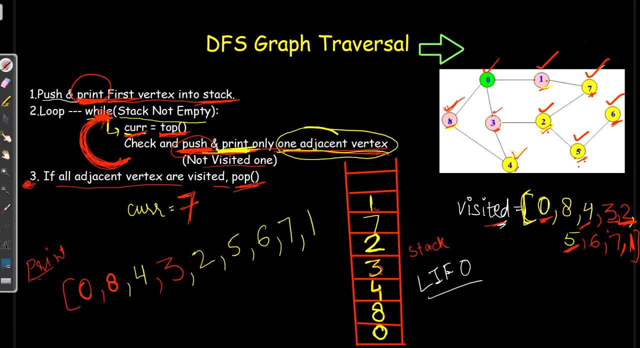 now. no, it is not empty. so it will take the topmost element one and will check its adjacent vertex for one. we have zero seven only, so zero seven are already visited. so if all adjacent vertex are visited, pop it. so here i will pop one. then again it will go to while loop is stack empty. no, so i will take. 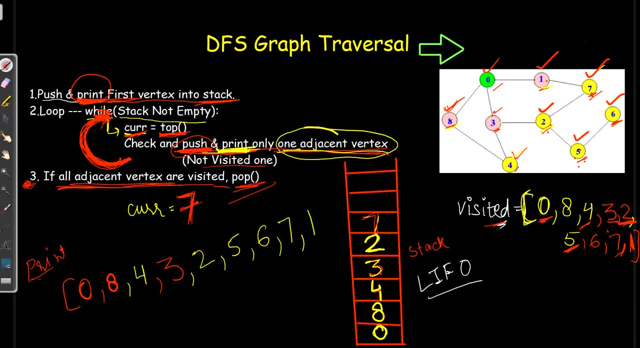 the topmost element, seven. seven adjacent vertex are one and two. one and two are already visited here as we have here, so i will pop seven. then again it will go to y loop. it will take two here in current. so for two, three, seven and five are already visited. so if all vertex are visited, 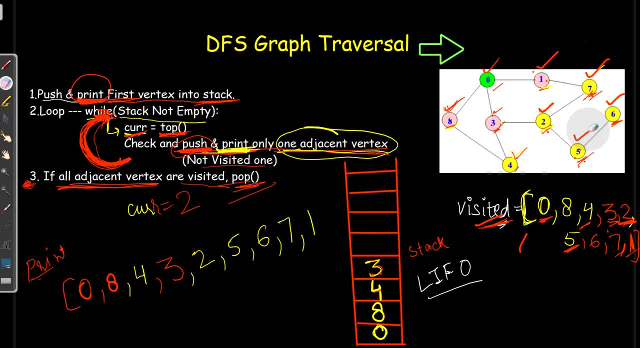 pop two, as all elements are visited. let's check out for three, for three, zero, four and five above and 2 are already visited, so i will pop 3, then 4, 4. we have 8, 3 as adjacent vertex, so they all are visited, so i will pop 4 here, then we will check for 8. 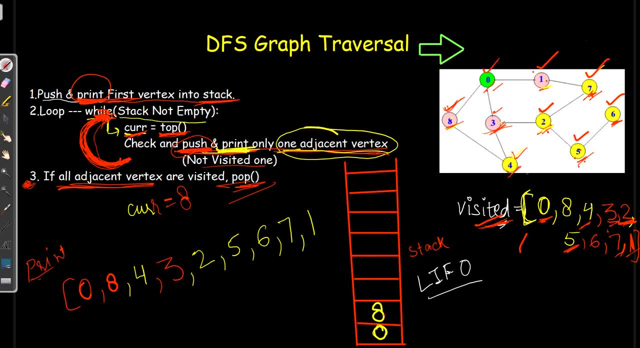 for 8: 0 and 4 are already visited, so we will pop 8 also. then for 0 we have 8, 3, 1 are already visited, so i will pop now again. it will go and we'll check whether stack is empty. yes, this time stack is empty, so it will come out and will print these elements, which is: 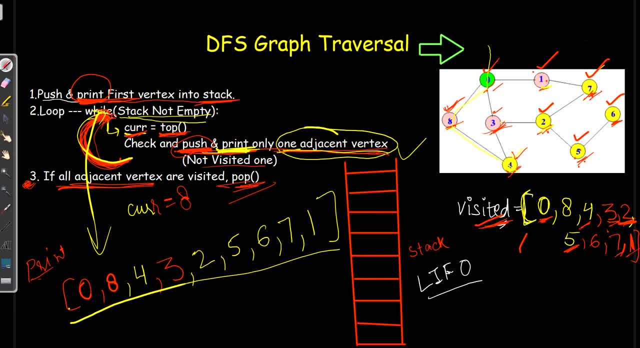 0, 8, 4, then 3, then 2, 5, 6, 7 and 1, so here it is printing vertically. so this was dfs, which prints in depth, which goes in depth first and then prints, and here we are making use of stack which works on lefo. let's check it out, its program also. so we will go to. 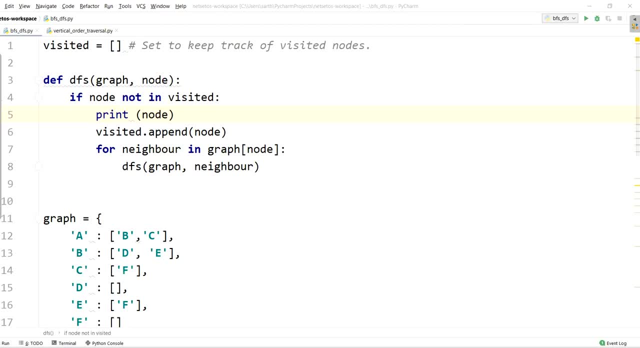 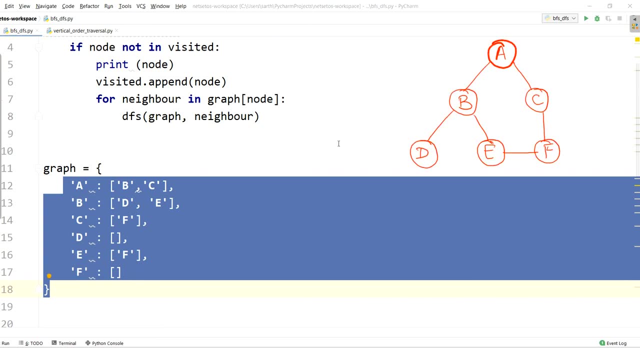 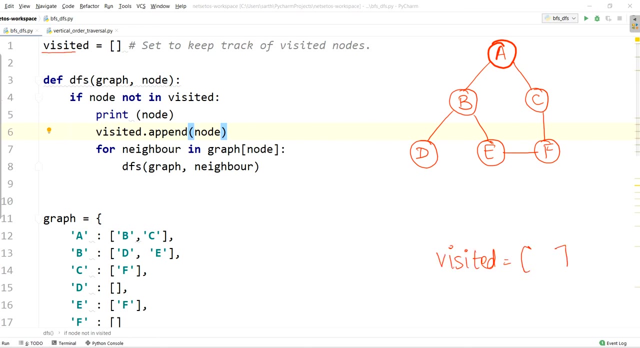 pycharm. so here we have the code for dfs. first of all, what i'll do, i'll plot this graph. the graph is same as the last one, so let's start. first of all, we have visited the empty array. then we will take graph and node as an input parameter. graph we have here and node the starting vertex, whichever vertex you. 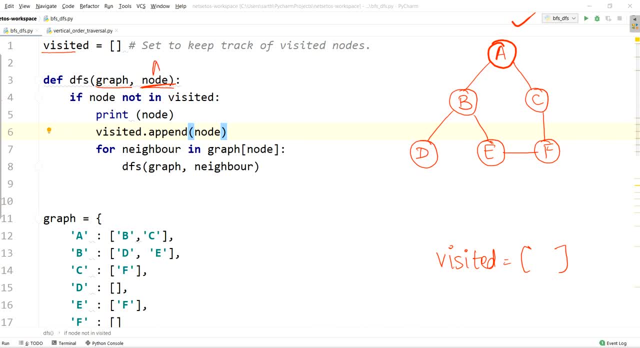 want to start. you can start with it here. i am taking a for my starting vertex. now we will check for a, whether a is there in visited array. so this code is completely unrecursion. if you face any problem in recursion, i have a complete playlist on recursion for you. 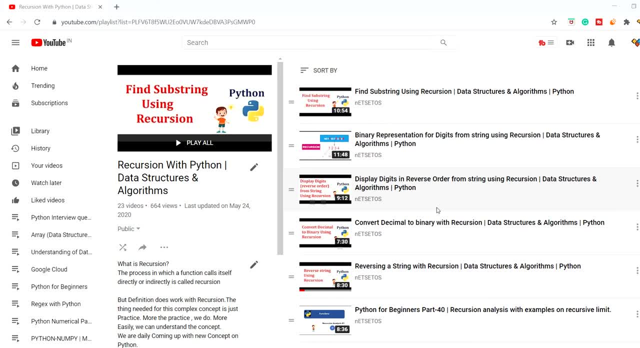 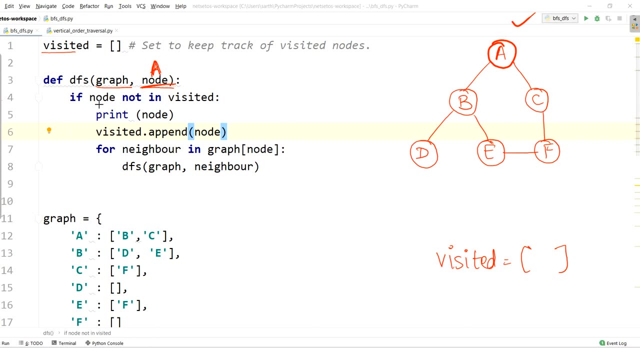 here i have explained recursion elaborately so you can go for it for understanding recursion in a more clear way. so i'll recommend you to go for it and understand recursion in a very simple way. so back to our question. here we have node a which will check in visited array whether visited. 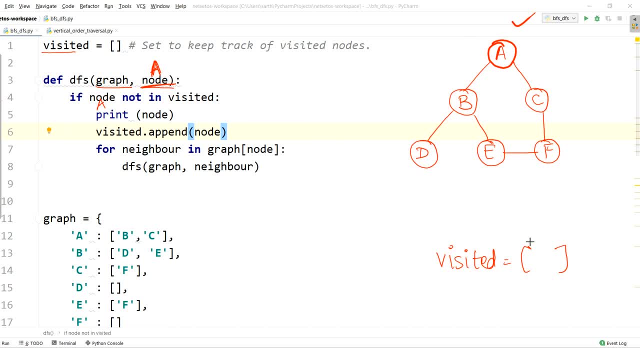 array has a here visited array is an empty array so it will go inside if condition and will print a over here and will have a in our visited array. s a is now visited, then it will go and check for neighbor a. a has two neighbors, b and c, here. we need to take just one neighbor, as i told you in. 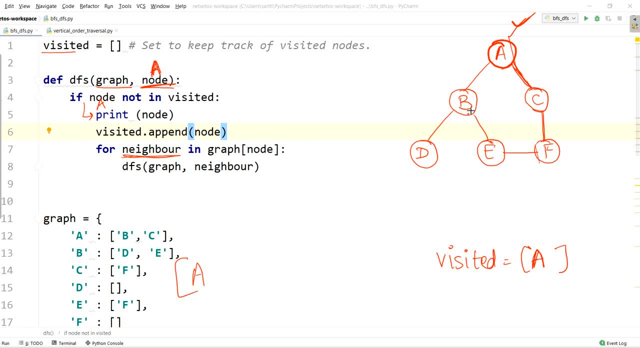 algorithm. we have option. we can take any of them. Here I am taking B, So we will check for B. For B is there in visited? No, it's not there. So it will go and will print B over here and will have B in visited array. So let's make it visited Then for B it will check its neighbor It has. 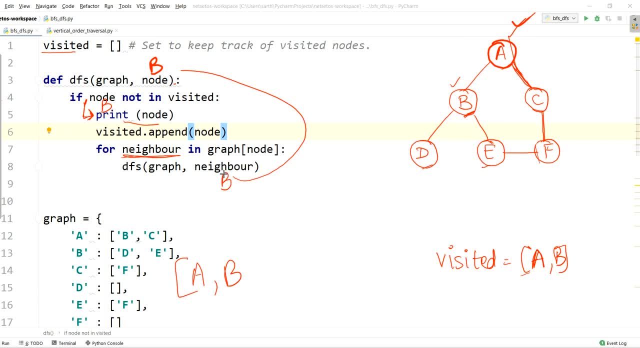 D and E. We can take either one of them. So I will take D over here. So it will check pericursively: D is there in visited array? No, it's not there. So it will print first and then will append in visited array. Then it will check for D neighbor Whether D has. 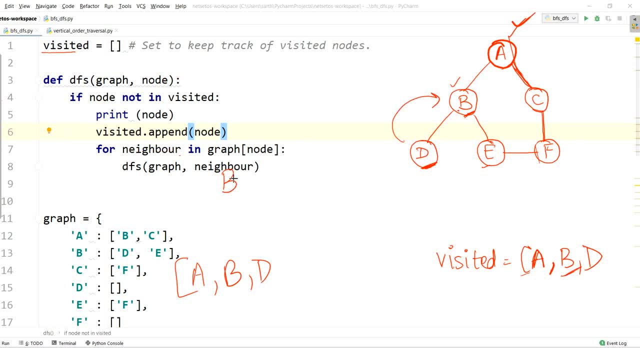 neighbors. it has B, So for B it will check. It has D and E, So this time it will take E and will go recursively for node is equal to A and will check whether node not in visited E is not there in visited, So it will print. 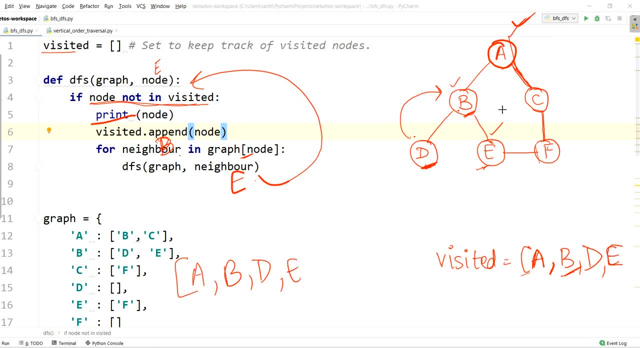 first and will have in visited. Now for E, it will check its neighbors. It is B and E and F. B is already there visited, So here it will have F. So for F it will check whether F is visited. No, it's not visited, So it will go inside if condition and will print F and 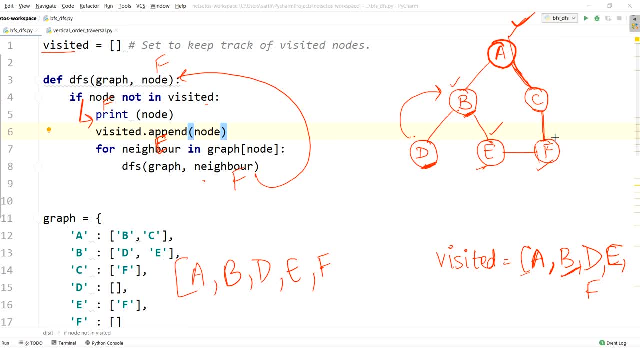 visited array will have F here, So let's make it visited. Then for F, E and C: E is already visited, So it will check for C now. So here we have node as C For C it will check. it is there in visited No, So here it will print C and will append C in the visited array. 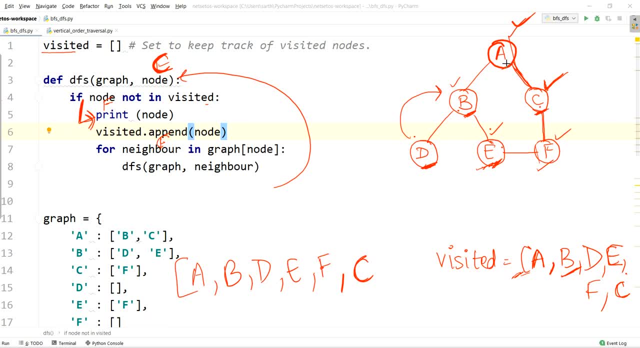 So here with C is the visited one. Now for C, A and F are the neighbor which are visited one. So here we will get A, B, D, E, F, C as DFS. Let's check it out. So I'll run the code here I. 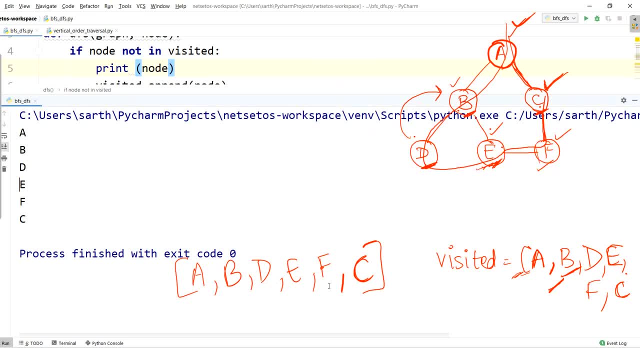 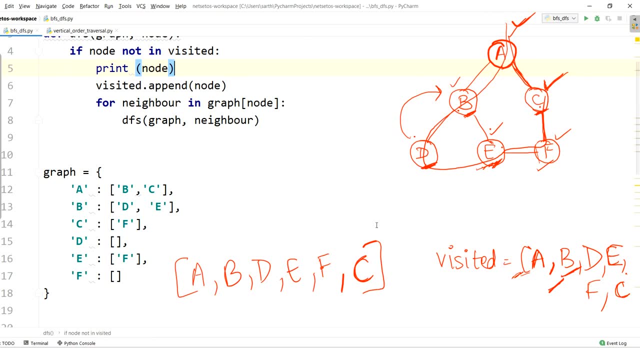 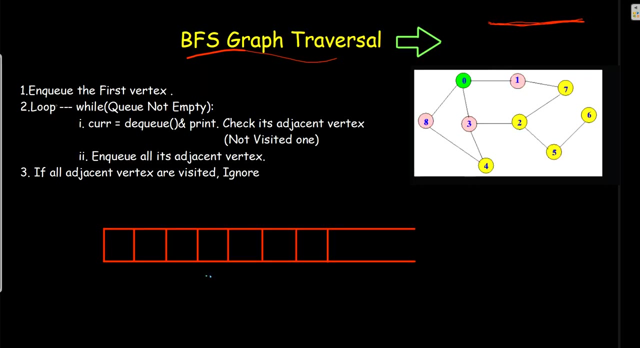 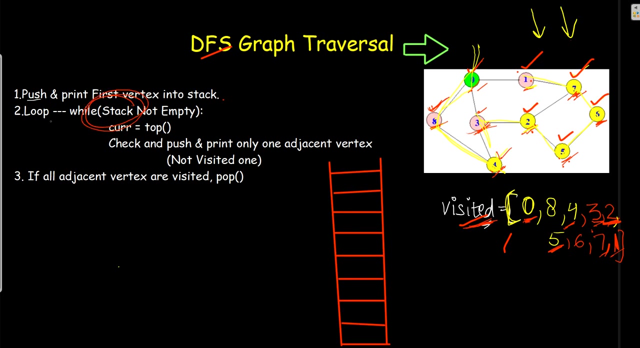 got A, B, D, E, F, C as my printed array. So this is all about DFS- depth first search. Here we made use of stack, Now BFS with DFS. in BFS we made use of Q, while in DFS we made use of stack in BFS.